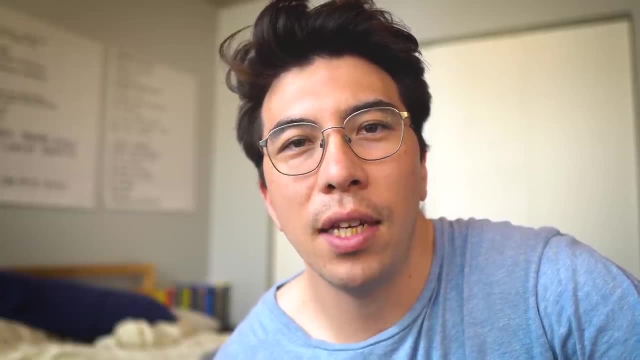 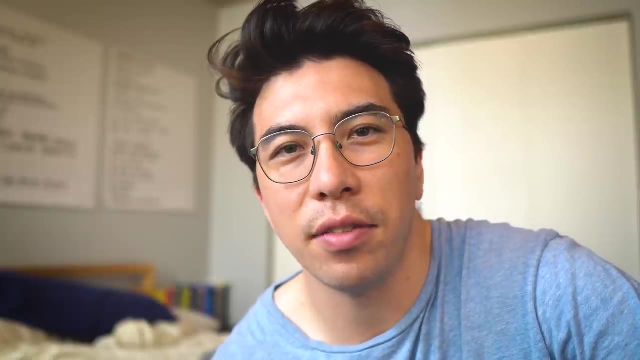 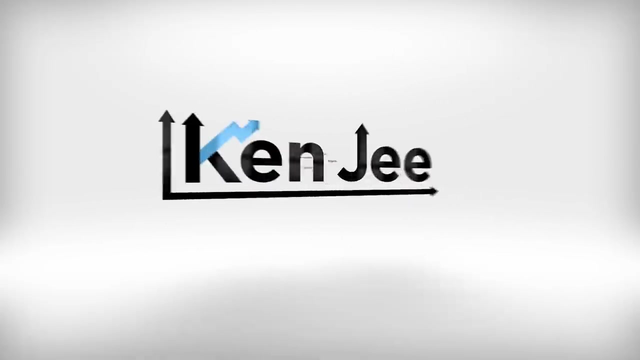 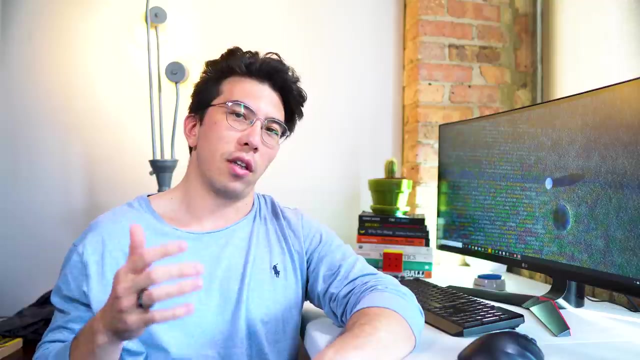 data scientist positions. In this video, I'm going to go in-depth into the responsibilities that each of these different roles have and how they differ across the data science lifecycle. Before we talk about each of these positions, I think it makes sense to describe the data science project lifecycle. The main difference between 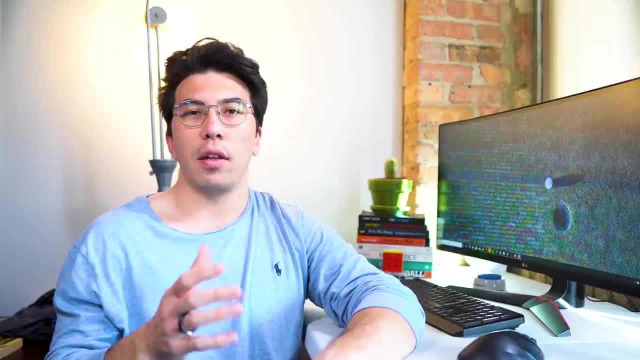 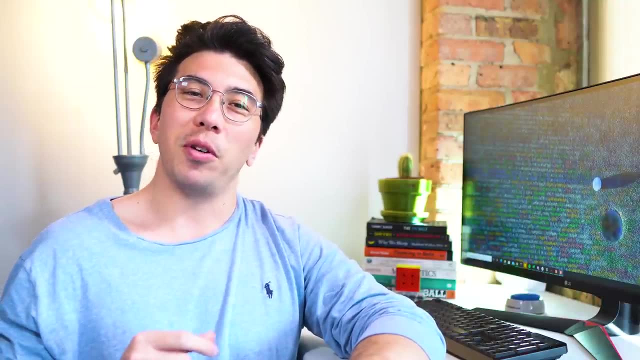 these roles is the areas of this lifecycle that they cover. If you enjoy this content, please hit that like button. Also, please subscribe and turn on notifications to be alerted when I post my next weekly video. As it turns out, you need actual data to do data science. so the first step of the 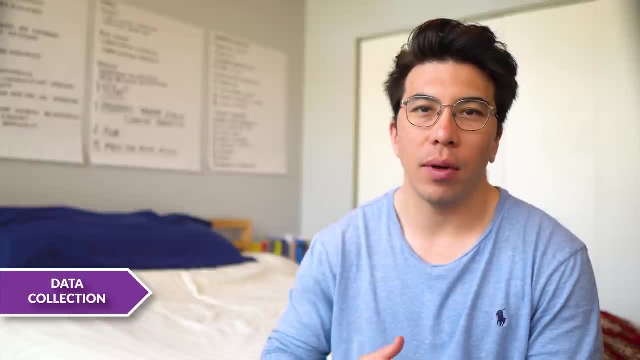 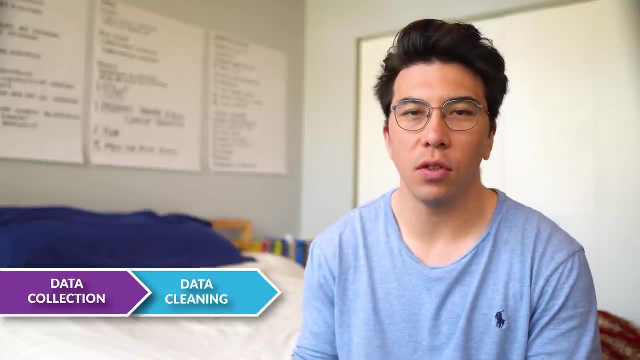 data science lifecycle starts with the data collection. This is where we aggregate and store data. The next part of this lifecycle is the data cleaning. We need to make sure that this information is usable and stored in a way that's easily accessible. Usually, we access it through structured query. 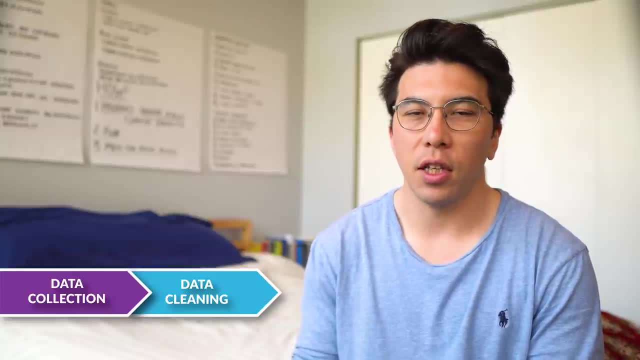 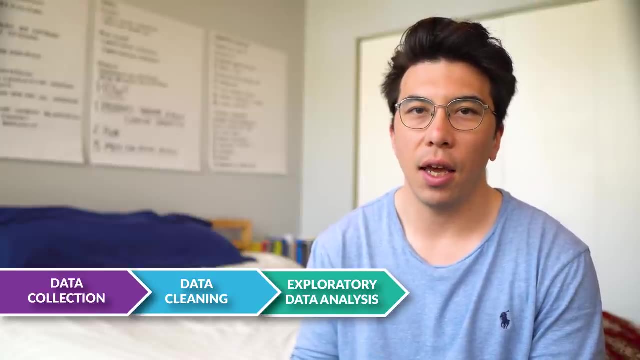 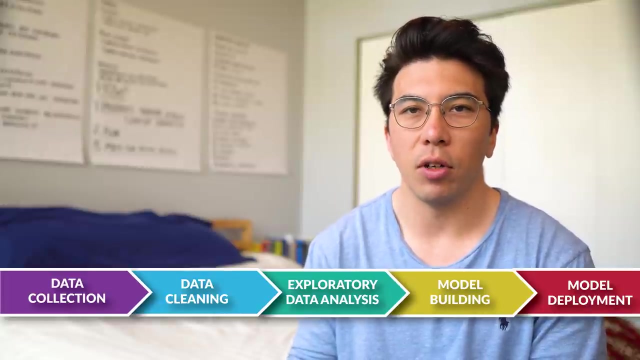 language otherwise known as SQL. Next comes the exploratory analysis. In this step, you look for trends and high-level insights from the data. It's also known as EDA, and it's followed by the model building phase. This is where we try to predict outcomes from our analysis. The final step is model. 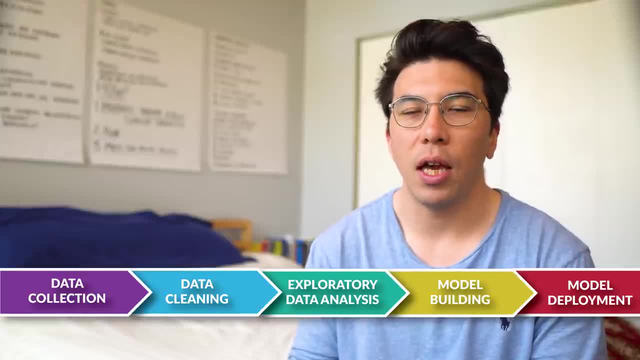 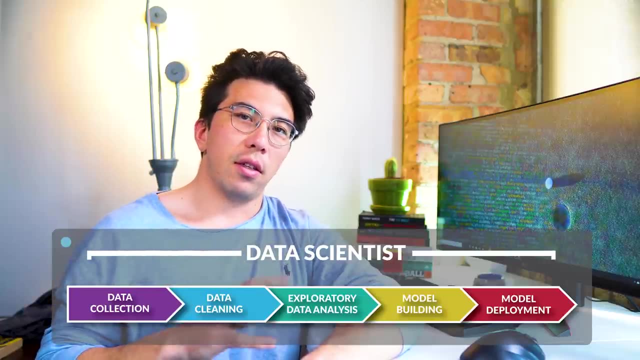 productionization. We take our machine learning models that we built and we make them scalable for the business. The traditional data science role broadly covers this whole lifecycle. Data scientists can also specialize in some areas of this pipeline. I personally work more on a data cleaning EDA and 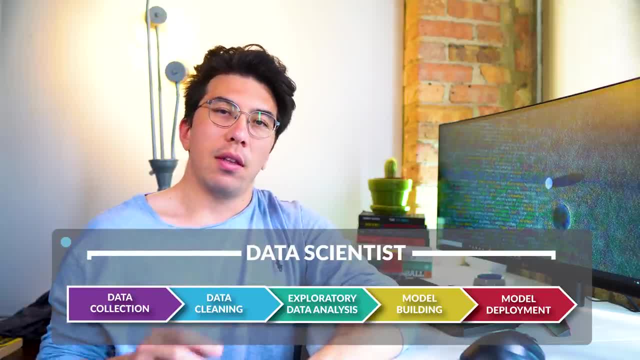 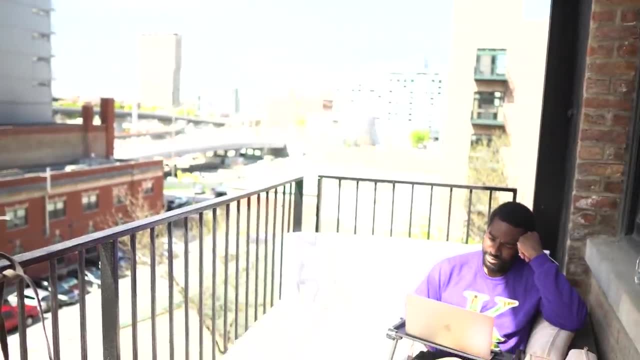 model building than any other part of the spectrum. The data science role has has the most flexibility across this life cycle and what you do in the role can vary greatly by the company you work at, because of the broad description data scientists can be expected to do. 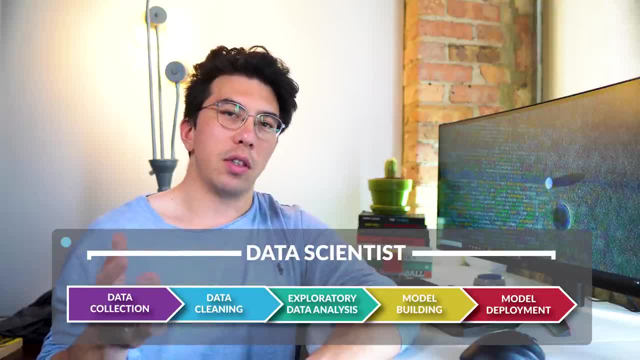 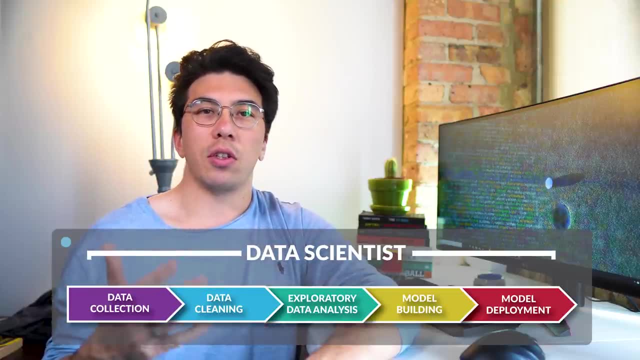 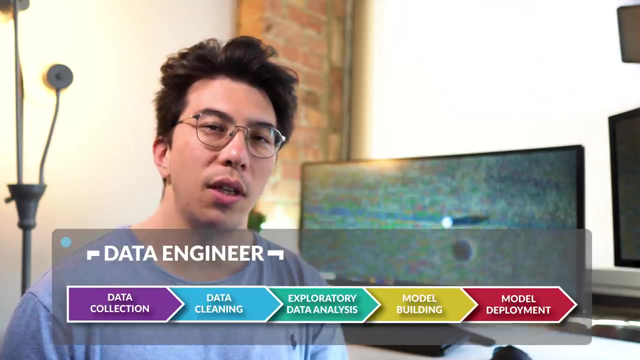 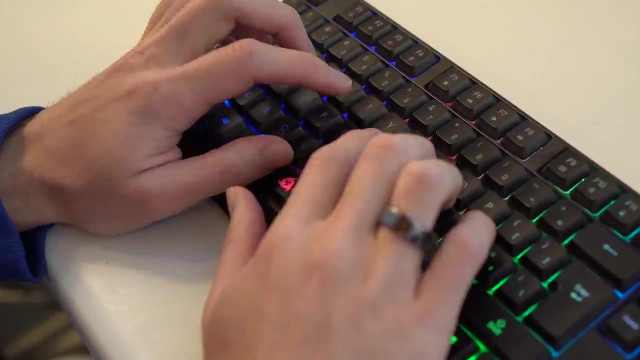 anything from data collection, like web scraping using sql, to query databases, programming in python and r, building machine learning models and also creating productionization pipelines in flask or aws sagemaker. the data engineer role usually focuses on data collection and data cleaning. in this position, you're expected to have a very strong grasp of sql. you'll be pulling data and